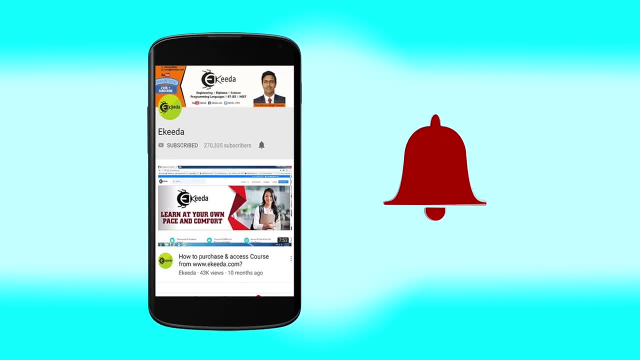 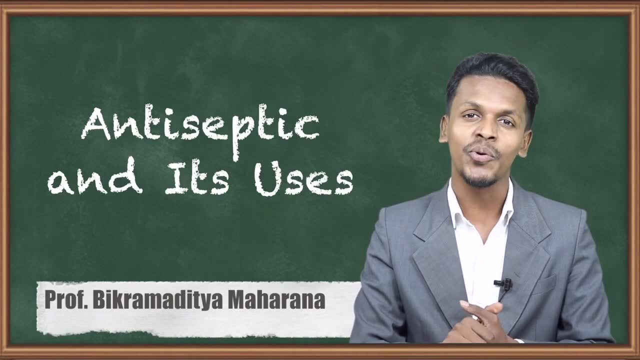 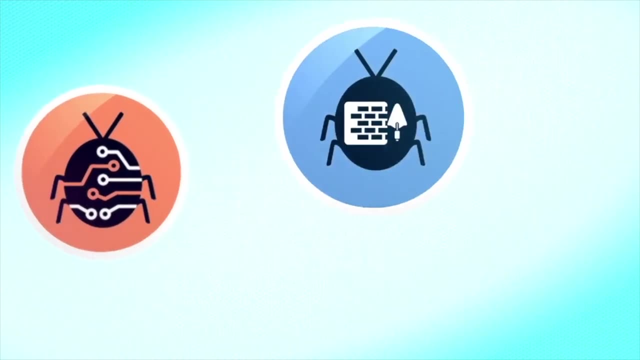 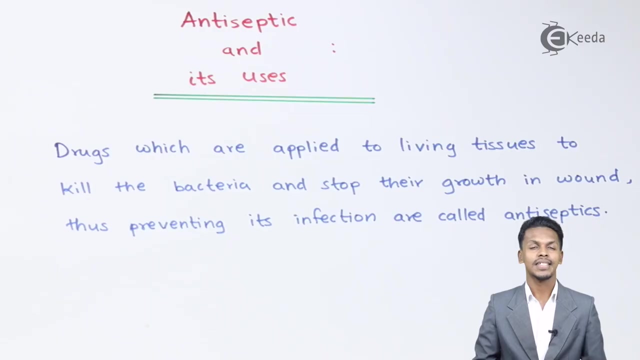 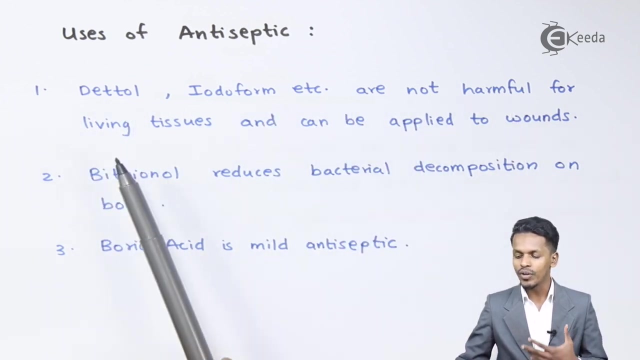 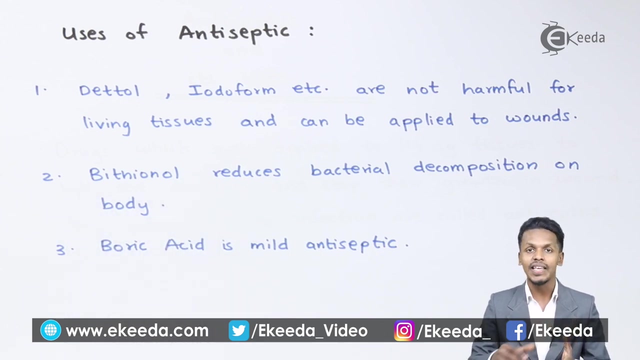 Click the bell icon to get latest videos from eKIDA. Thank you for watching. Thank you for watching. Thank you for watching. This is what the uses of biothanol is, and this is what it is present in the soaps, or either it is present in the form of that is. 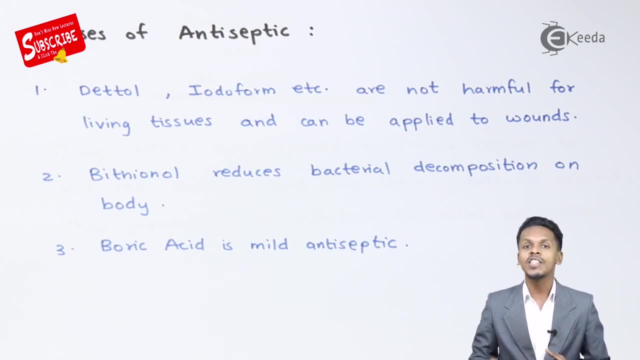 So talking about the other use, that is, boric acid. So boric acid is in fact a mild antiseptic and most of the swimmers- that is, professional swimmers- they use boric acid in the form of erotron Because the water in which they are basically swimming so that could be infected because of the microorganisms and all. 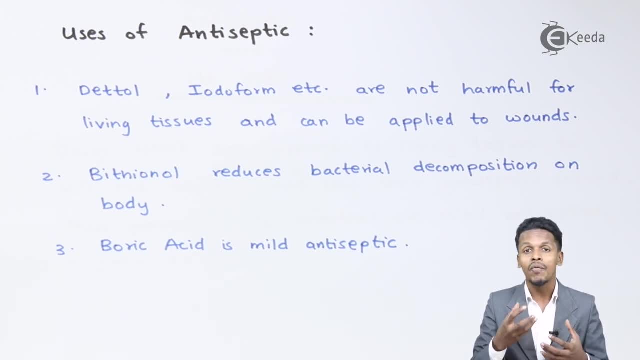 So that would be polluted water, So they have a chance that the fungus could grow in their ears. So to avoid that thing, so they are using boric acid. So boric acid can be used as eardrop, but not only eardrop, but they can also use it in the form of an eye wash.